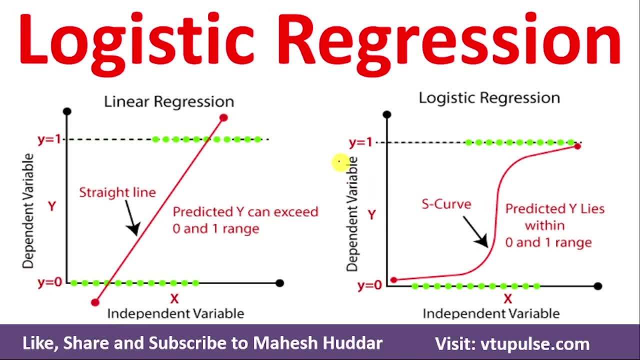 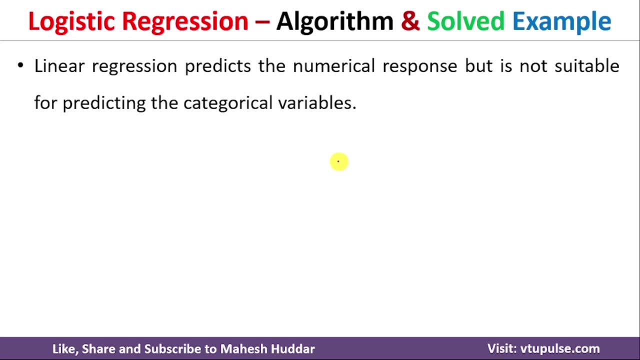 Welcome back. In this video I will discuss logistic regression algorithm in machine learning with a simple solved example. In the previous video I have discussed linear regression and polynomial regression with a simple solved examples. Linear regression model is used whenever we want to predict the numerical responses, That is, if the dependent variable 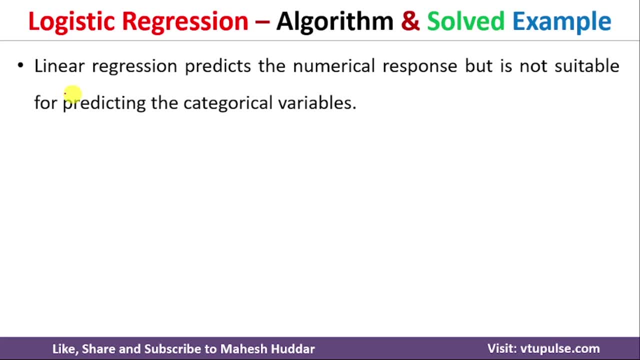 is of type numerical or continuous. in such cases we will use either linear regression or polynomial regression model. But if the response variable is of type categorical in nature, then we cannot use a linear regression model. If the dependent variable is of type categorical. 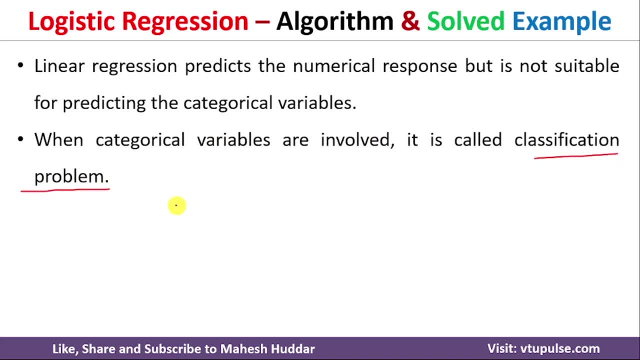 such kind of problems are called as classification problems, And these kind of problems can be solved with the help of logistic regression. And this classification problem should be of binary nature, That is, if the class or the target variable contains two possibilities, then we can use the logistic regression. if we have more than two possibilities. 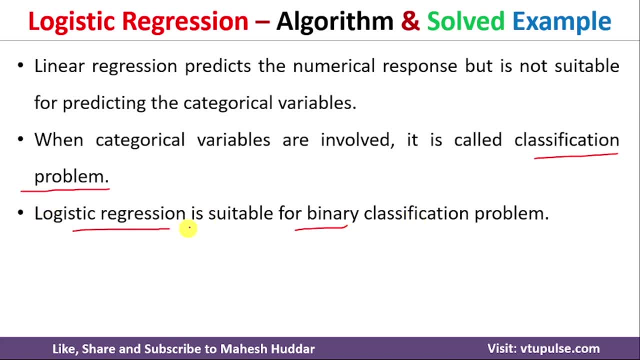 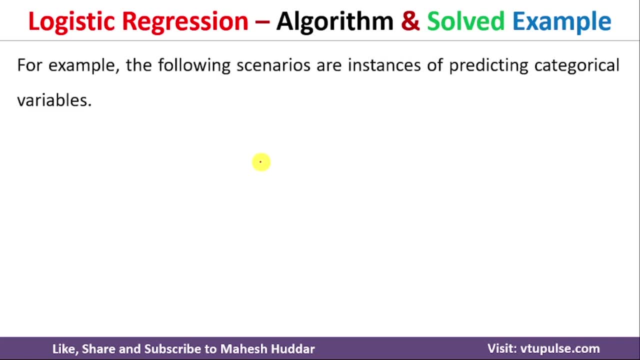 in classification or the target, then we cannot use logistic regression. before we proceed with logistic regression, we will consider some of the classification problems. let us say that we want to predict whether the given mail is spam or not spam. in this case, the class is binary nature, hence 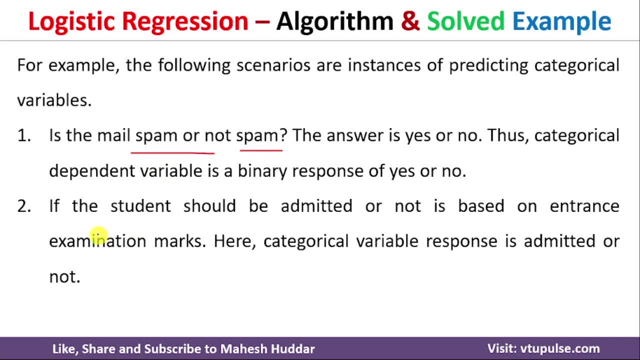 we can use the logistic regression over here. the second example is whether the student should be admitted or he should not be admitted, based on the entrance examination marks. in this case also there are two possibilities. are there whether the student should be admitted or not admitted? again, we have two possibilities. hence we can use logistic regression here. in the third example: 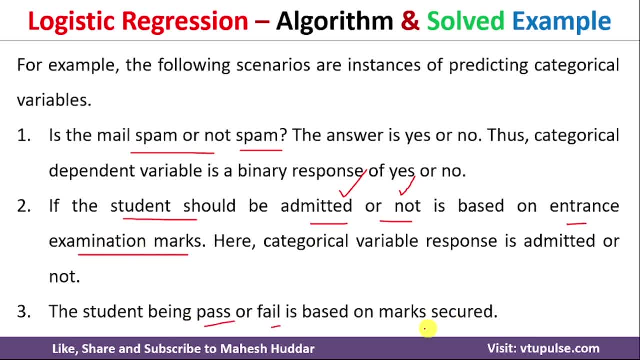 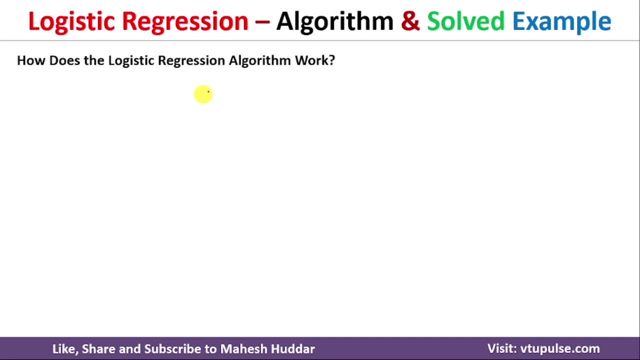 whether the student will pass or fail in the examination based on the marks secured. that can be predicted with the help of logistic regression, because we have only two possibilities here. now. the next question comes in front of us is how the logistic regression works, how the logistic regression algorithm works. to understand the logistic regression algorithm, 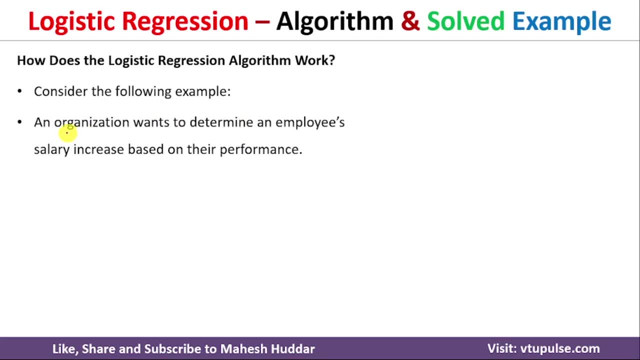 we will consider one example. let us assume that the organization wants to determine an employee's salary increase based on the performance. that is what should be the hike given to that employee based on his performance. if you want to know this particular salary hike, what we can do over here is: 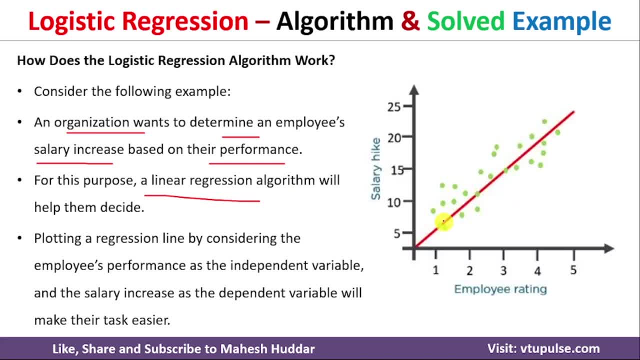 we can use a linear regression algorithm, that is, we will plot the employee rating against the salary hike. the employee rating is independent variable here and the salary hike is a dependent variable. so once you plot this particular point, we need to find a line which will fit to this particular given. 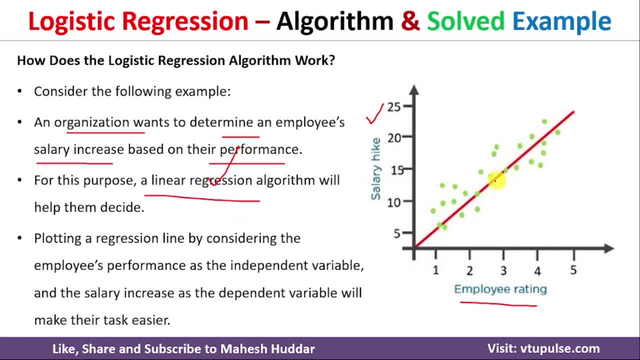 data with the help of linear regression model. once you get this particular linear regression model, based on this particular employee rating, we can easily get the salary hike here. for example, let us say that the employee rating is one he will get around five percent of, we can say that salary hike. 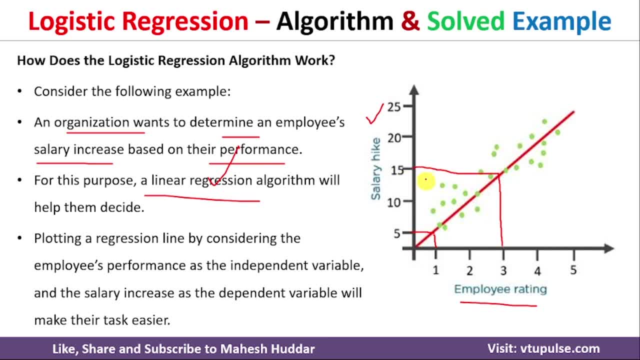 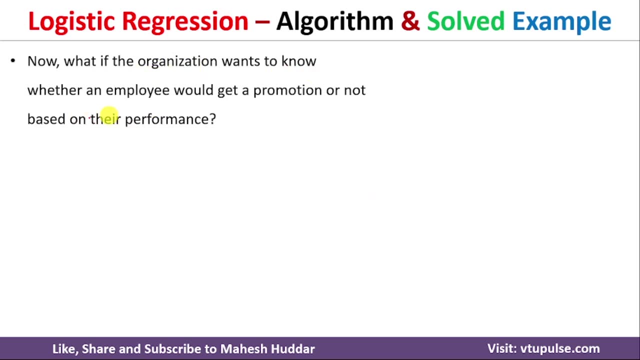 if the employee rating is 3 over here, he will get around 15 percent of salary hike. if it is you can say that 4 over here, he may get around a 20 percent or a 17 or 18 percent salary hike and so on. but let us assume that the organization wants to know whether employee should be given. 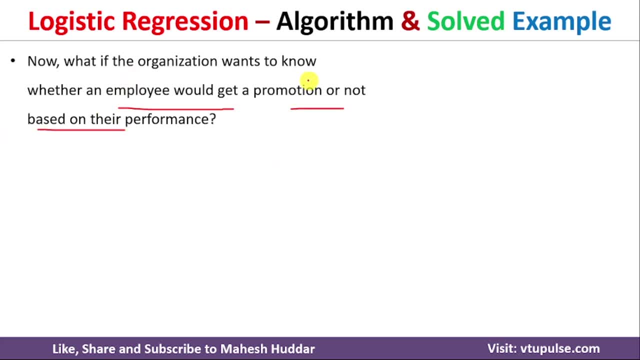 promotion or should not be given promotion. so in this case we have only two possibilities: whether the promotion should be given or promotion should not be given. in such cases, the linear regression model won't help to solve such kind of problems, so here we need something called as the sigmoid. 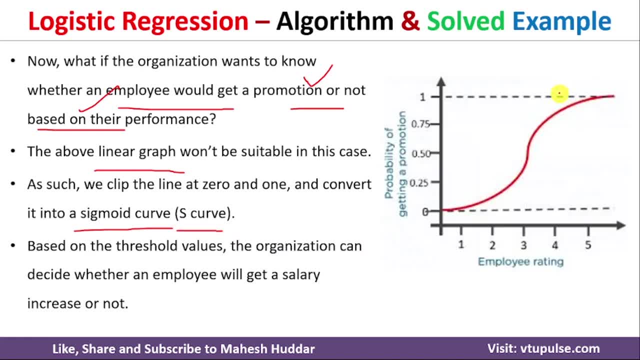 curve, or also called as the s curve, which looks something like this. so, based on the employee rating, we want to find the probability of getting promotion here. in this case, we are going to find the probability of getting promotion and based on that particular thing we will decide whether. 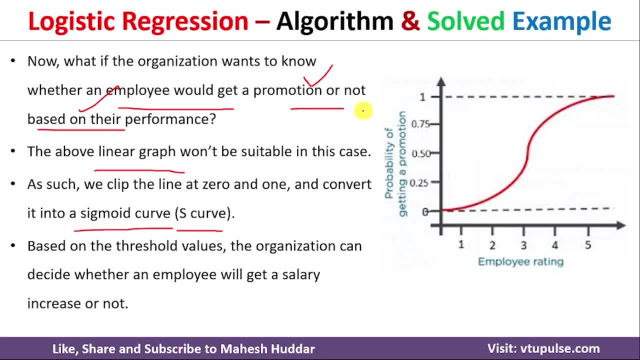 the employee should be given promotion or should not be given promotion over here. let us say that we will calculate the probability. the probability will be always in the range of 0 to 1. over here the calculated probability is 0. so in such cases what happens over here is the person may not be given promotion over here and if the calculated 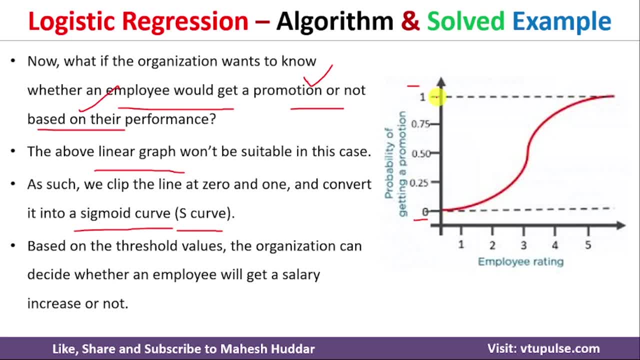 probability is 1, the person will be given promotion for sure. now we cannot get 0 and 1 all the time. there is a possibility that for this particular person, the person with the employee rating 3, the we can say that probability of getting promotion is around. i can say that 0.3035 or something like that. 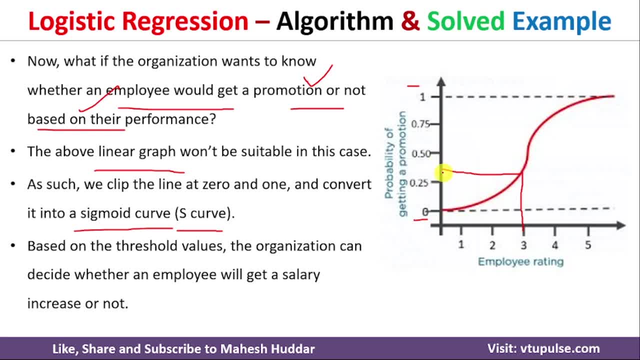 now what? what will happen here? whether the person will be given in promotion or it will not be given a promotion. the same thing happen with respect to this also, let us say that 4 and if you go and draw this particular thing, the probability of getting promotion is 0.75. here again, whether it will be, 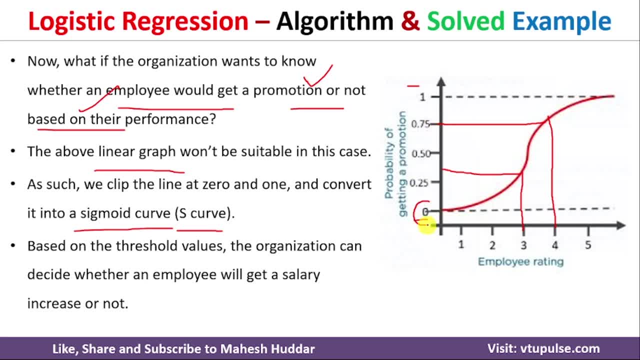 given or not. that's a question. as i said earlier. if the probability of getting promotion is 0, he will not be given promotion. if it is 1, for sure the promotion will be given. but what about these? or for? what about the values in between 0 to 1? in such cases, we need something called as. 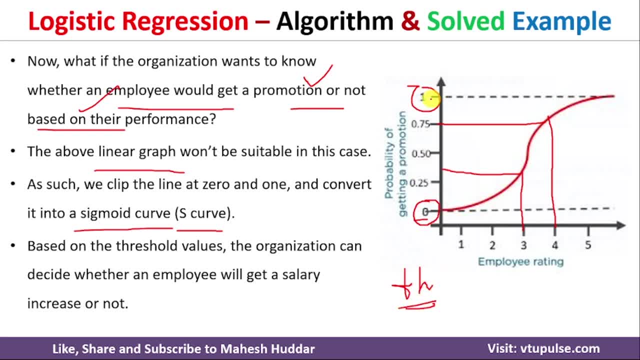 threshold over here. based on this particular threshold we will decide whether the promotion should be given or not. let us assume that the threshold is 0.5. if the calculated probability, that is, the probability of getting promotion, is greater than 0.5, the person will be given. 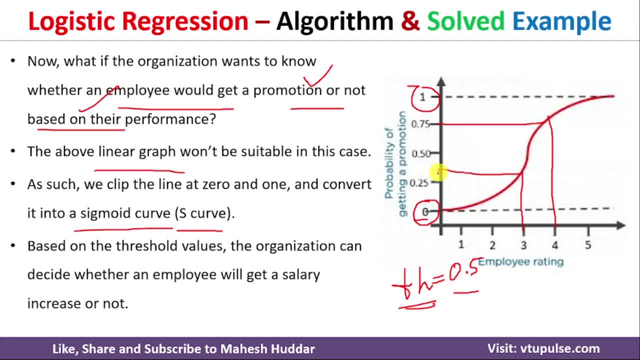 promotion or will not be given promotion. over here. for this particular person with the employee rating 3 will not be given promotion because it is less than 0.5 over here. for this particular person with the employee rating 4 will be given promotion because his probability of getting. 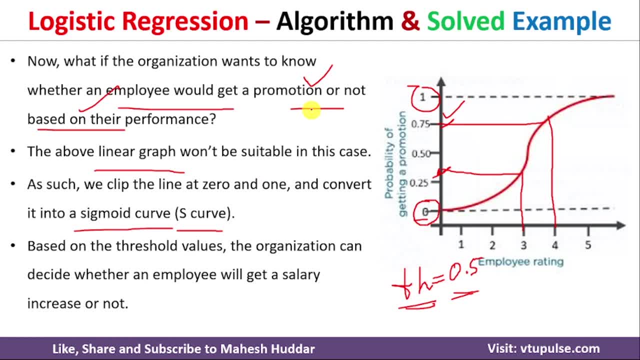 promotion is 0.75 in this case. so this is how the logistic regression algorithm works over here. so what we need to do is we need to draw this particular sigma curve, given that particular data set, and, based on that particular probability, we have to decide whether, uh, the new example should. 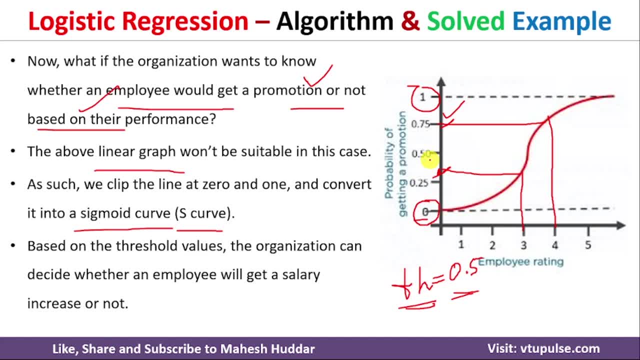 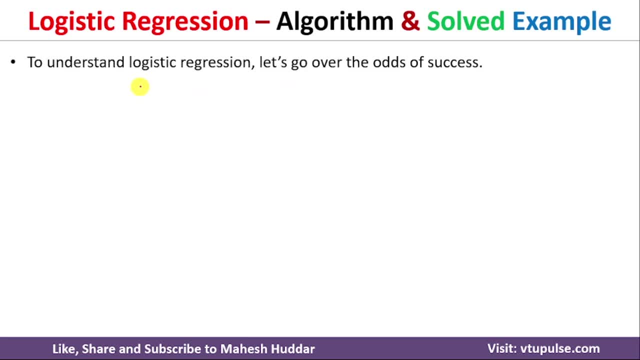 be classified into one class or another class in this particular case. over here now we will try to understand the mathematical concept behind the logistic regression. to understand the mathematical concept first we will try to understand odds of success. the odds of success is always equivalent to probability of an event happening divided by probability of an event not happening. let us say: 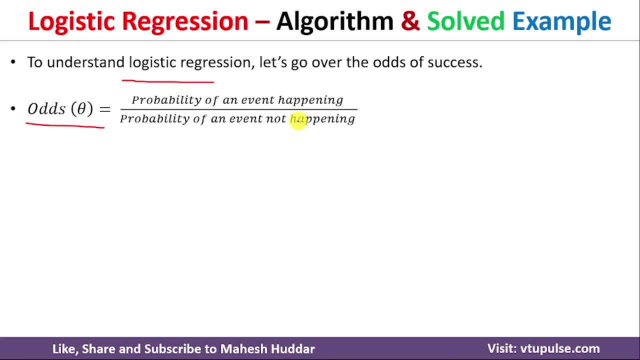 that the probability of an event happening is p, then probability of an event happening not happening is 1 minus p over here. so that can be written something like this: now what will be the possibilities of odds of success here is, the probability will be always in the range of 0 to 1.. if it is equivalent to 0, 0 divided, 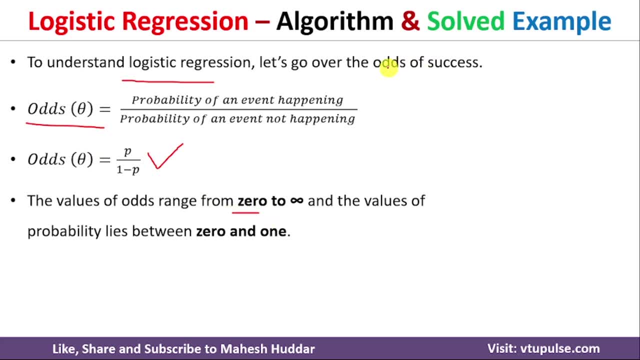 by anything is 0, so the probab odds of success is equivalent to 0 in this case, if probability is equal to 1, 1 divided by 1 minus 1, that will be 1 divided by 0. anything divided by 0 is infinity. 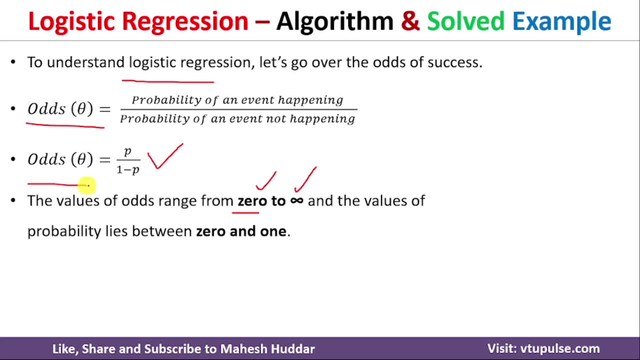 odds of success will become infinity in that case. so the odds of success will go from 0 to infinity, because the probability will always be there in the range of 0 to 1. in this case, We will consider one more equation over here, that is the straight line equation. 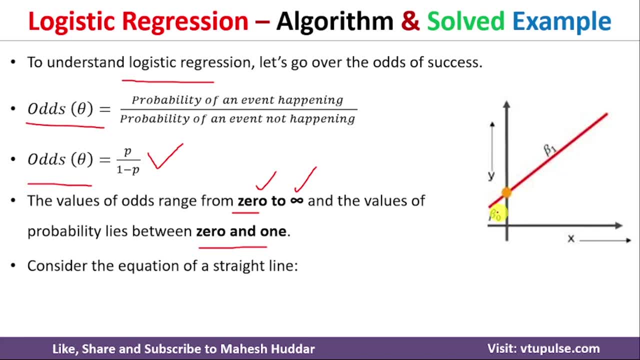 This is the straight line equation. as and when the x increases, the value of y increases. based on this particular, you can say that beta 0 and beta 1.. Here beta 0 is the intercept and beta 1 is the coefficient of x. over here. Now, this is how the equation for straight line looks like. 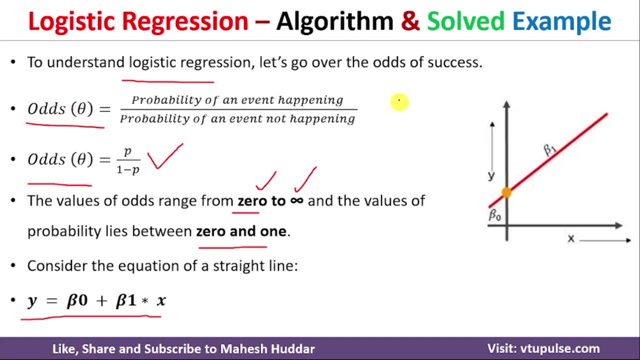 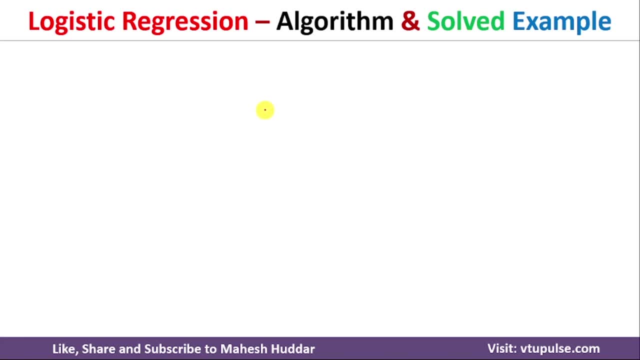 Now, what we do over here is, if you want to know the odds of success, we need to take the logarithm of this particular thing. So for that reason, what I will do here is I will take the logarithm on the left hand side of this one, that is, the odds of success. the logarithm of p divided. 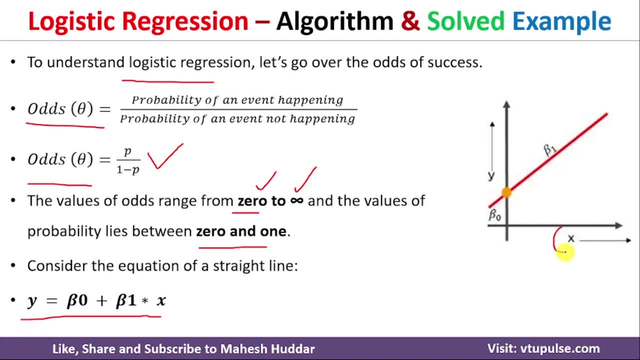 by 1 minus p. According to this particular diagram, I want to know probability of this particular x over here, happening of x, and then we will get the value of this particular y over here. So that is the reason. logarithm of probability of x divided by 1 minus probability of x is equivalent to y. 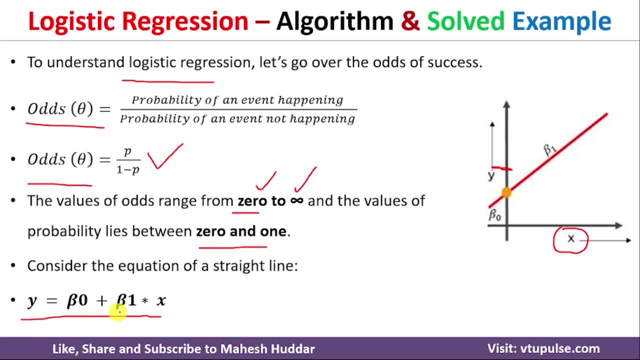 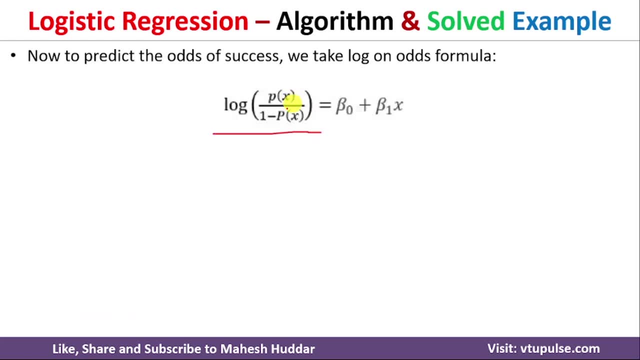 over here. So that will be the case. and y is known to us. that is beta 0 plus beta 1 multiplied by x over here. So the equation can be written something like this: log of p of x divided by 1 minus p of x, that is, the probability of happening of x divided by. 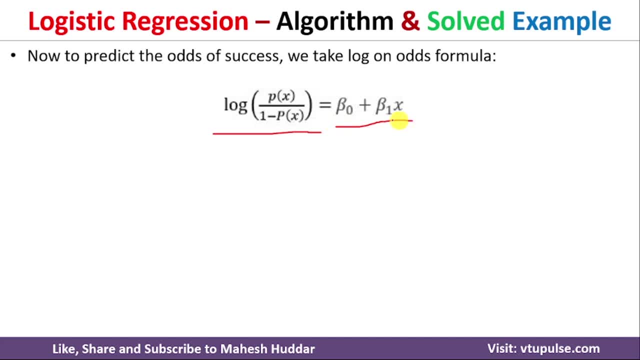 probability of not happening of x, which is equivalent to beta 0 plus beta 1 x over here. Now again, this particular formula doesn't look quite easy to solve. So what we do over here is we will take exponential on both the sides over here. So e raised to ln of this particular term. 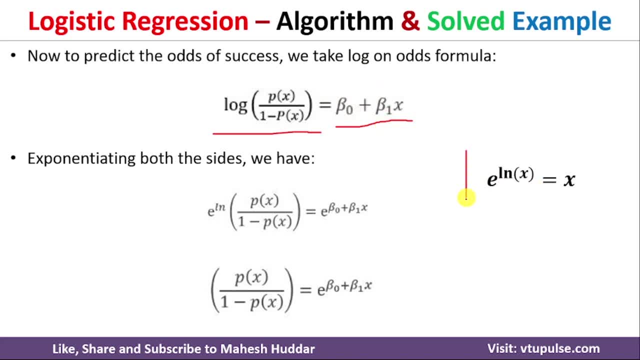 is equal to this particular term over here. Now we know one standard formula, that is: e raised to ln of x is always equivalent to x over here. So in this case, e raised to ln of this term is equivalent to this particular term over here, which is equivalent to e raised to beta 0 plus beta 1 x. 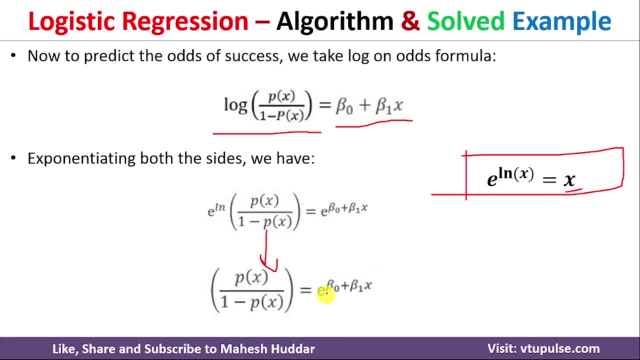 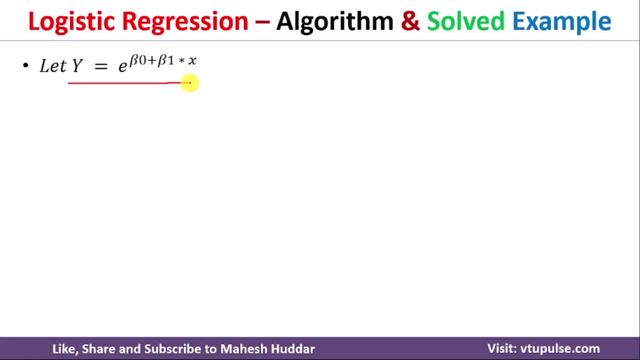 over here. Again, this particular thing cannot be solved so easily. So what we do over here is: we will set this particular thing is equivalent to y over here. So that is what I have written here and what we do here is, if I take e raised to b, 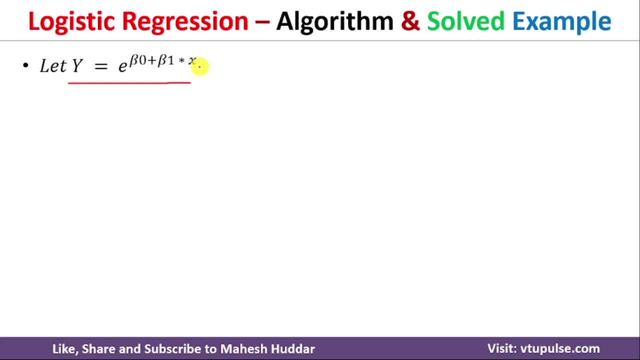 0 plus beta 1, x is equal unto y. now, uh, left hand side, we have p of x divided by 1 minus p of x, which is equal unto y. so this is how, actually, we will get the equation. now we will try to solve this one. we will take this on the right hand side. it will look something like this, and then we will: 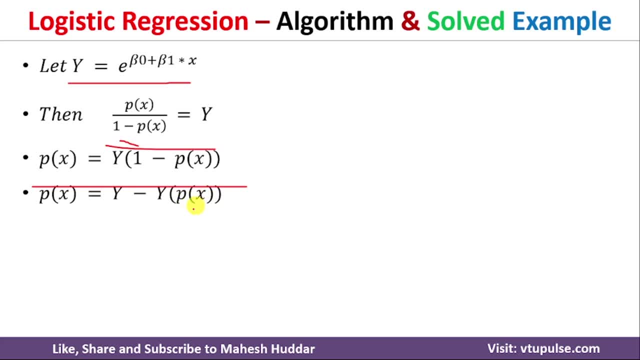 multiply it inside, we will get y minus y of px. we will take this one on the left hand side. it will look something like this: now we will take p of x. outside, we will get p of x. 1 into 1 plus y is equal unto y over here. so probability of x is equal unto y divided by 1 plus y over here. 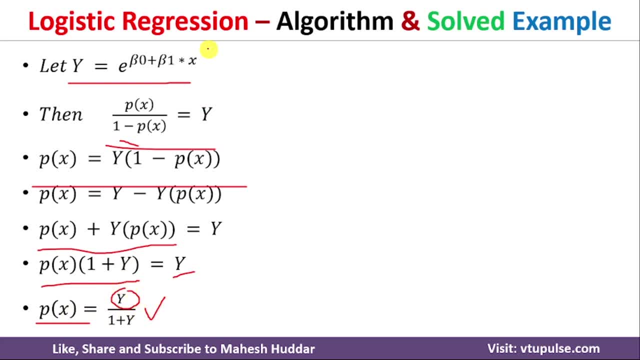 so probability of x is equal unto. we need to replace this particular y by this one, so we will get: probability of x is equal unto. e raise to beta 0 plus beta 1 x divided by 1 plus e raise to beta 0 plus beta 1 x. over here. now we need to simplify this particular term one more time. 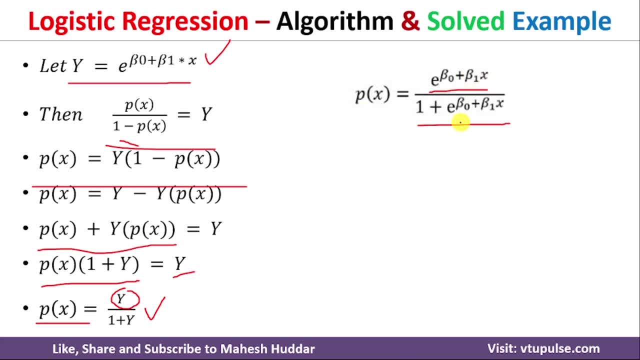 what we do over here is so we will divide the numerator and denominator by numerator over here, so this will be again the same term. whatever we have on the numerator e raised to beta 0 and all divided by this particular e raised to beta 0, we can say that beta 0 plus. 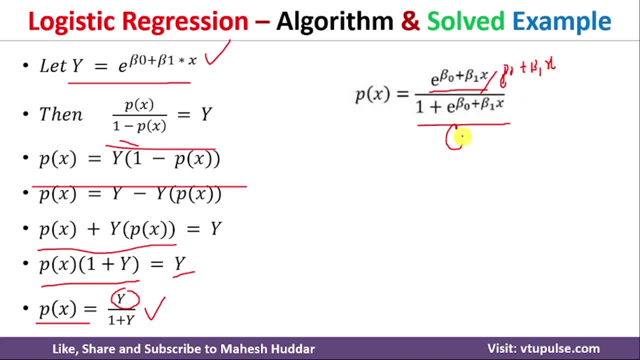 beta 1 x here. the same thing will come over here also. that is e raised to this one is beta 0 plus beta 1 x over here. now this particular term and this one will get cancelled. we will get what is that called as 1 on the numerator here and denominator 1 divided by this term plus this. 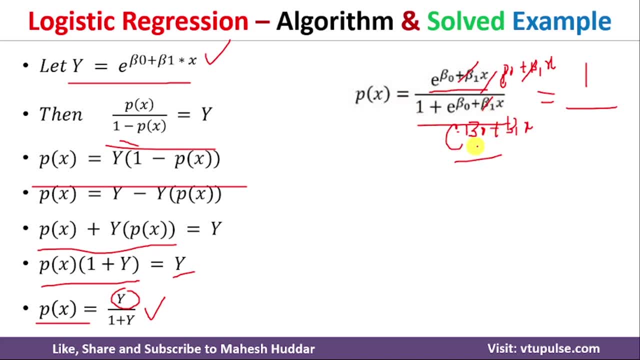 divided by this term. so this one and this one will get cancelled on the second one. but 1 divided by this one, that is e raised to beta 0 plus beta 1 x, that is nothing but e raised to minus beta 0 plus beta 1 x and e raised to beta 0. beta 1 x divided by this one is nothing but what 1 over here. so 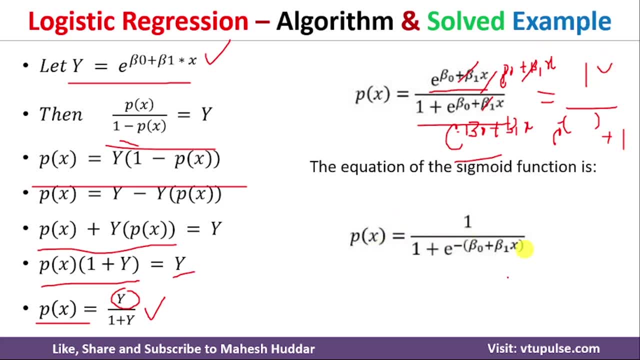 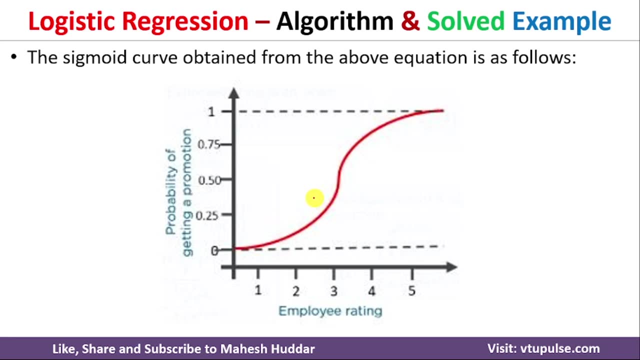 that is nothing. but p of x is equivalent to 1 over here. this one, i have written it here. e is to minus beta 0 plus beta 1 x. this is nothing but the sigma term over here. so because this is a sigma term, we will definitely get the s shaped curve, or it is also called as the sigma curve, over. 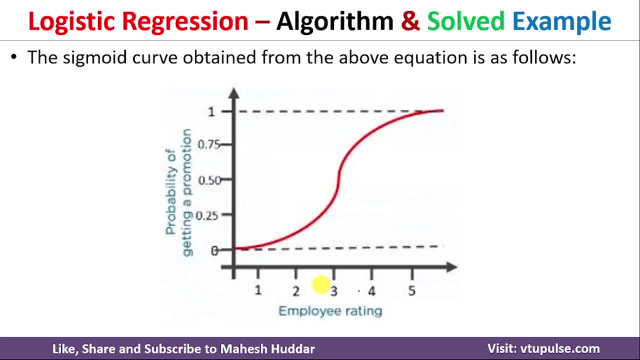 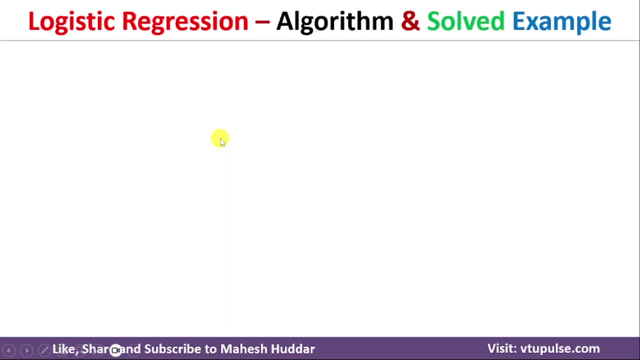 here and once you get this particular sigma curve based on this particular independent variable, we can easily predict the dependent variable over here. now, to understand this particular logistic regression, we will take one numerical example. let us assume that we have been given the student data set, that is, historic data set. who are selected or not selected in this particular case? 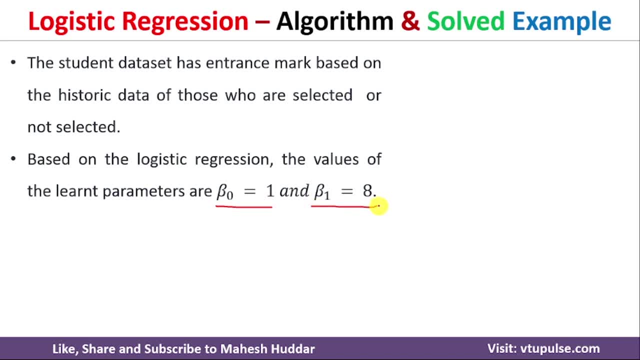 what is given to us is the beta 0 value is given and beta 1 value is given. also, the x value is given over here. so given this particular x, we need to compute whether that particular student will be selected or will not be selected over here. 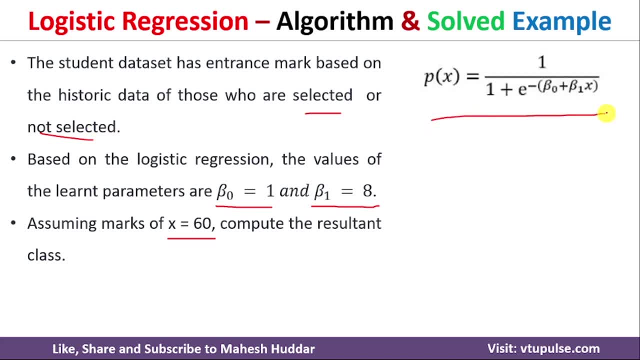 so we know the equation for that particular student logistic regression, that is, p of x is equal to 1 divided by 1 plus e. raise to minus beta 0 plus beta 1. x. beta 0 is known to us, beta 1 is known to us, x is known to us. so first we will solve. 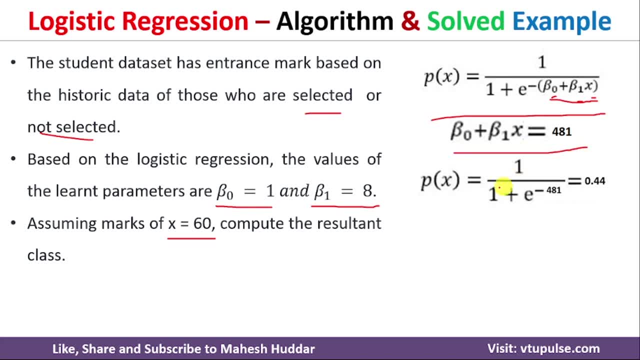 this particular term, that will become 481 over here. the meaning of this one is: p of x is equal to 1, divided by 1 plus e raise to minus 481, and if you solve this particular thing, you will get 0.44 over here. now what we need to do is we need to decide whether that particular person will be. 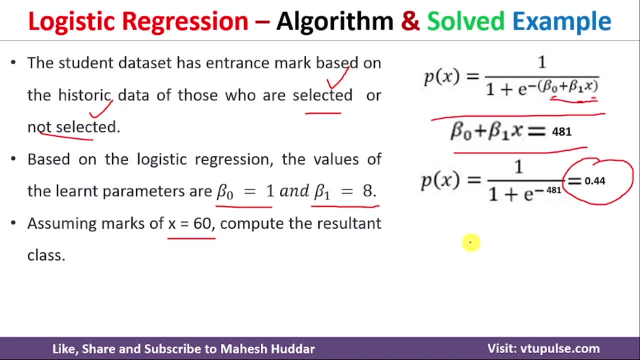 selected or not selected. so for that reason we need to know the threshold. assume that the threshold is equivalent to 0.5. the calculated probability is less than 0.5. the meaning of this one is: with marks 60, the person or a student will not be selected for in the entrance examination. 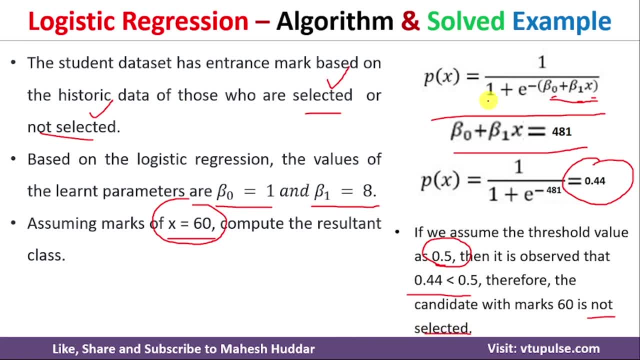 over here. so this is simple decision we can make based on the calculated probability as well as the threshold over here. in this video i have discussed what is the difference between linear and the logistic regression. so in this video i have discussed what is the difference between linear and logistic regression. also, i have solved a numerical example and discussed how to make a